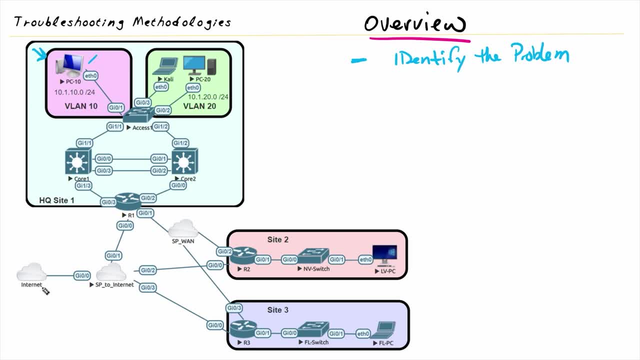 is that this user, who normally can access the internet, can no longer access the internet. The second step would be to establish a theory regarding why that might be happening, And so, by leveraging a topology like this, we could ask ourselves a few questions, For example, 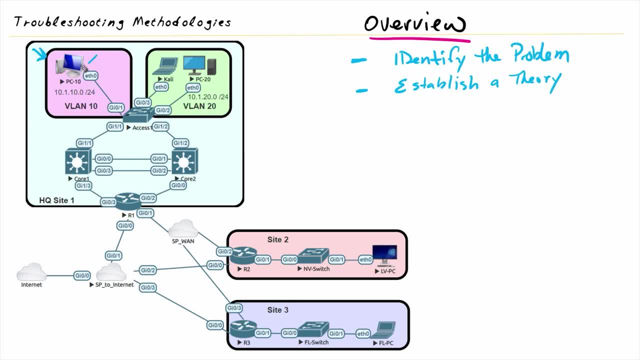 is this computer powered on? If the computer is powered on, does it have an IP address? And if the DHCP client, did it get the right information regarding a default gateway and the subnet and all that good stuff? And then, regarding this port, is this port on the switch? 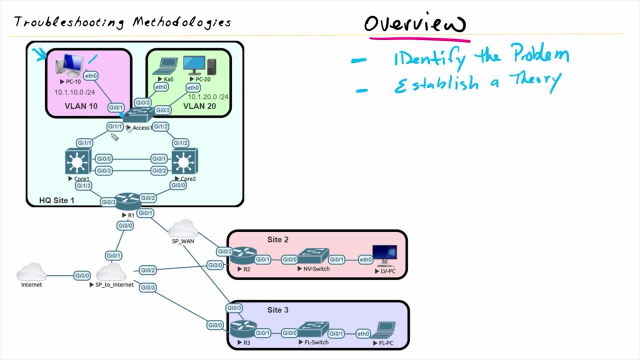 is it associated with the right VLAN, which is VLAN 10?? And regarding the trunking, is it going down from the access layer switch to the core? Is trunking working And is VLAN 10 being allowed? And then, from the default gateways perspective? 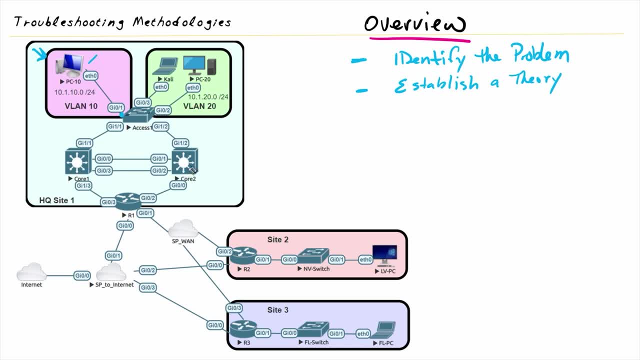 regarding VLAN 10, who's acting as the default gateway? Is it core one or core two, Or are they using a first hop redundancy protocol And, if so, which one of these two devices is acting as the active device, And does that device acting as the default gateway have a route? 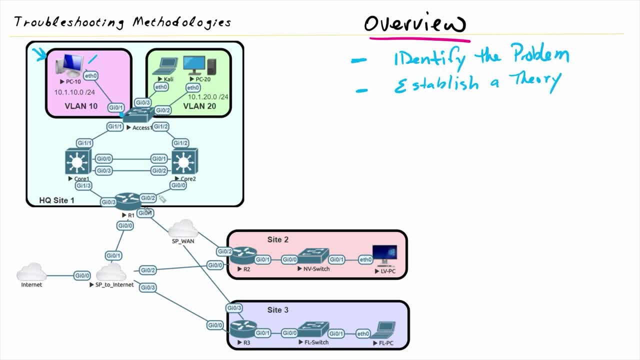 out towards the internet. In simple terms, does it know how to forward? And the same thing would hold true for this router and then this connectivity to our service provider. and also because we're using RFC 1918 addresses, perhaps network address translation is failing. 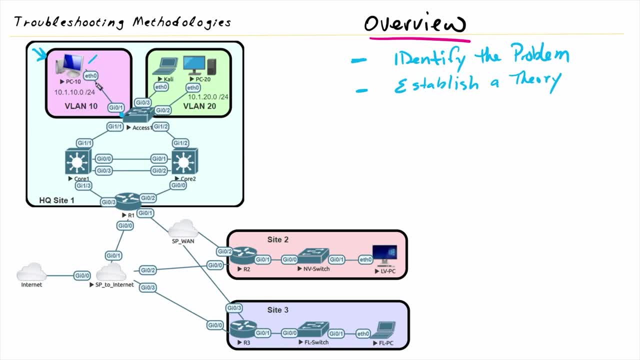 or isn't implemented correctly. So if this user at PC 10, by doing a few tests we verify that it can ping its default gateway And if this device in VLAN 10 up here at headquarters can ping devices out here at site two and site three and has reachability there, 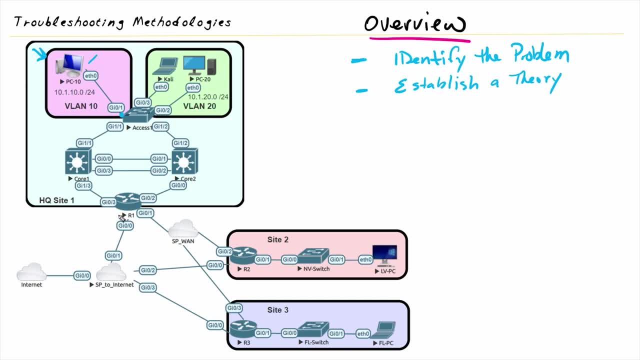 that can help identify what is working, And then we can establish a theory about what may be specifically causing the problem. And then, once we've narrowed it down to what we think it might be, and then the third step is to test, which is to basically go in. 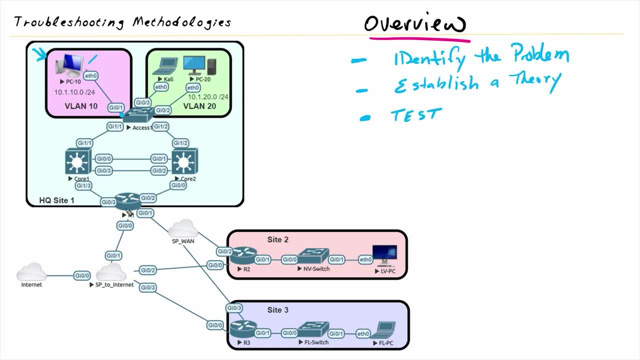 and prove your theory. If we think the problem is with router one, or if we think the problem was with the multilayer switch, or we think the problem is with the access layer, we want to do some testing to validate that what we think may be the problem really is causing the problem. And then 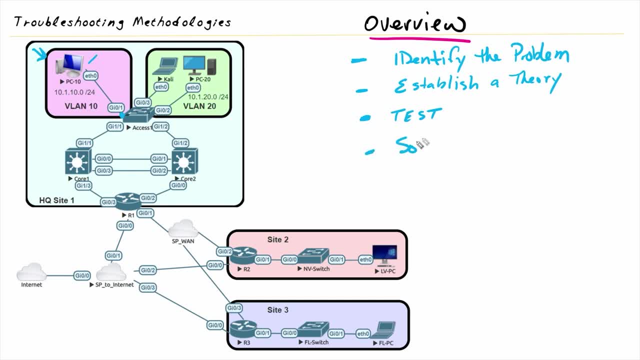 once we've narrowed it down and verified it, we then want to go ahead and solve the problem Now. solving the problem in an organization also has many steps involved with it. Let's list a few of those. as far as the solution to this network connectivity problem that the user is having, 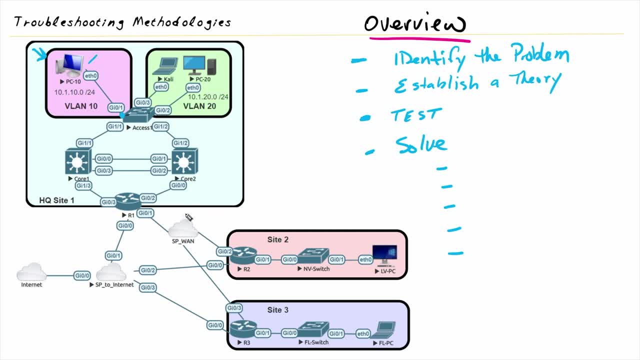 out to the internet. And let's also imagine, based on our testing, that we believe it's an issue with address translation, which could be NAT or PAT, but definitely needs to happen at some point before that traffic goes out to the internet. So if we've done some testing and we've narrowed it down, that 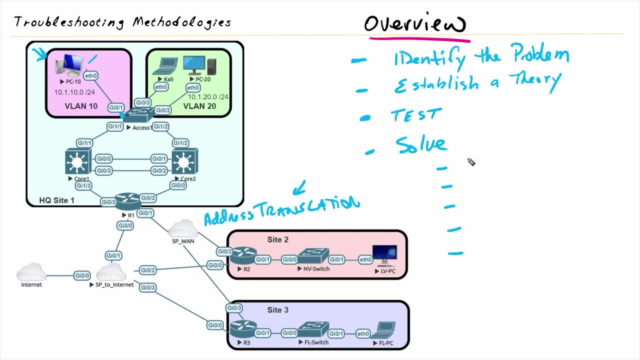 it is an address translation issue regarding solving that. we want to create a game plan on exactly how we are going to solve that problem, Perhaps with network address translation. the NAT device was set up to support VLAN 20 with the 10.1.20 subnet and other networks like this. 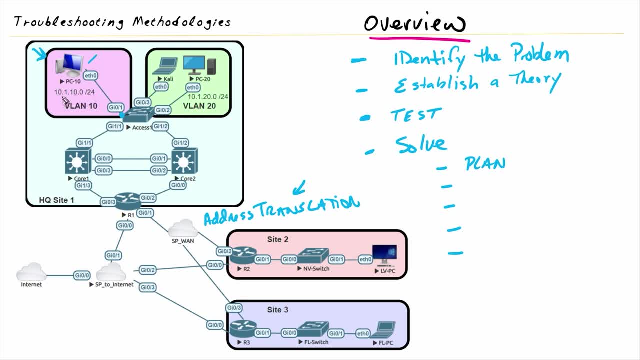 over here at site two and site three, But maybe perhaps not including the 10.1.10 subnet, So we'd want to make a plan to correct that. And also in corporations that's going to involve going through change control if we're going to make a. 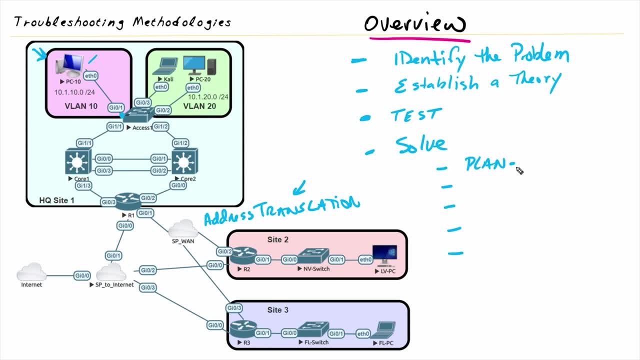 configuration change And then, with the authorization from the change control board, then we're going to go ahead and implement the change And then, when we've implemented it, we also want to verify that it's working, And that verification would involve a few things. Number one that we now have: 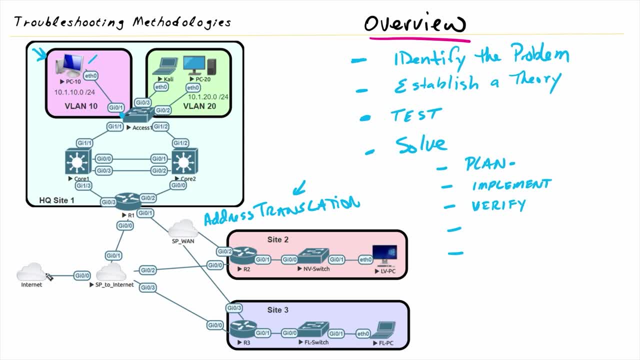 connectivity from this PC out to the internet. Also, we'd want to verify that we didn't make any other changes that would negatively impact our environment, Like we want to make sure that everything else still functions as well- VLAN 20 and the other. 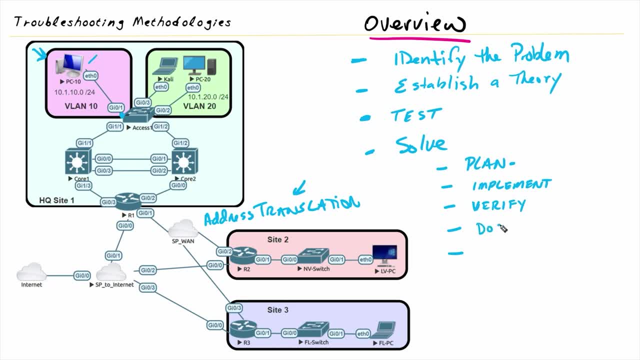 sites everybody can still forward out to the internet. And then we'd also want to make sure we document the solution, what we did, how we did it, And if we change the topology in some fashion, we'd want to include that update in our documentation. So the documentation of what, 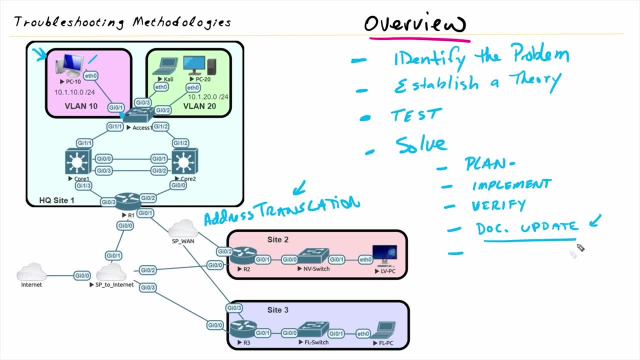 was done and also the topology, if there's been updates. that's super important because, let's say, three or four days go by and we have yet another problem And we think, oh, I wonder if what we changed here injected additional problems into the network. So we 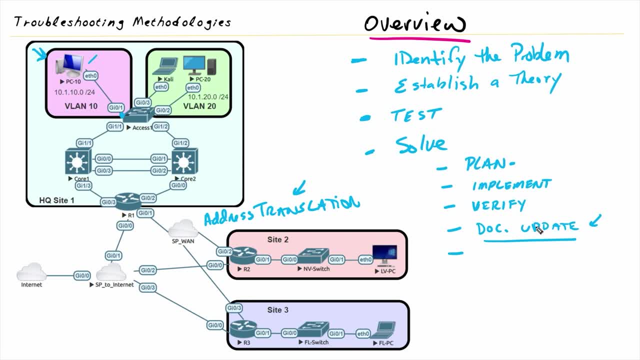 can go back through our paper trail and identify what happened when it happened, what was changed, And that can help speed up our troubleshooting, because a lot of times there are cabling issues and physical issues and so forth, But a lot of times when something breaks on the network, 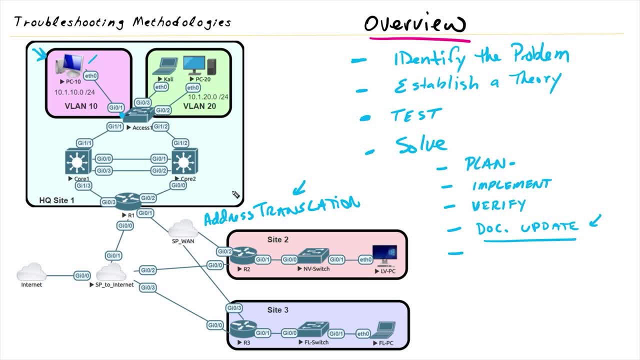 when something stops working, it's quite often due to the last change that was made, And so if we go back and take a look at the last change or two, that can help us reduce our troubleshooting time by either confirming that what was done is not impacting our current problem or by verifying 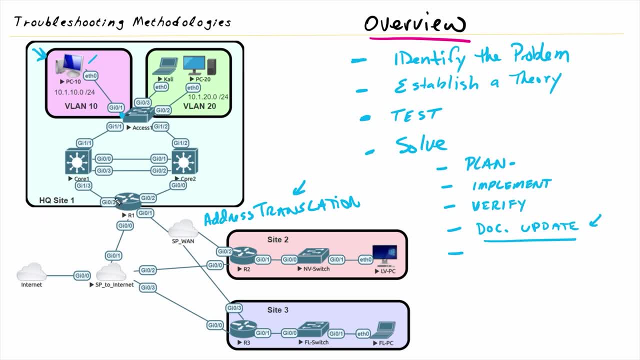 that what was done indeed is impactful. And then the last step here is to go ahead and repeat this process for the next problem. So the next service call that comes in, the next issue, the next problem. Again, we're going to follow this logical plan. So what I think would be fun to do is